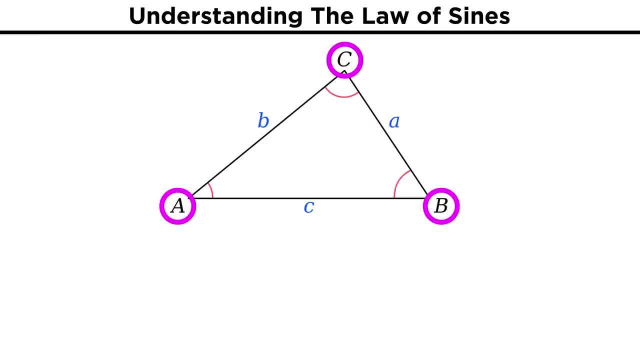 This law says that for an oblique triangle with angles A, B and C all capitalized, as well as sides A, B and C all lowercase, where the sides are precisely opposite their corresponding angles, The relationship between all of these will be: A over sine A equals B over sine B, equals C over sine C. This is: 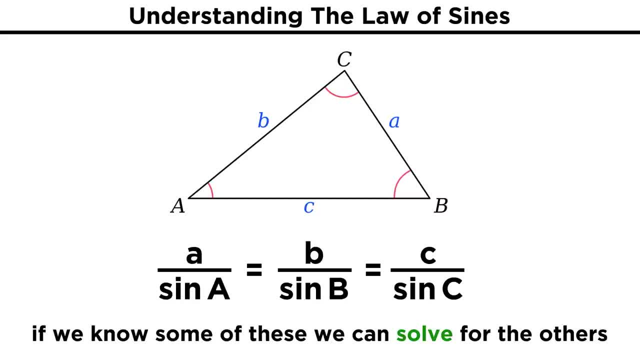 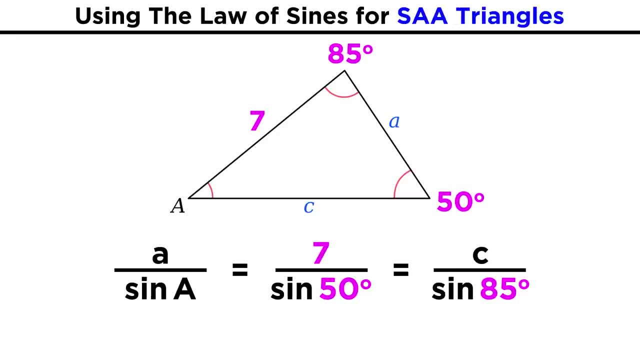 pretty easy to remember and not too hard to apply. We just have to know a few of these values and we will be able to solve. for the rest, Let's look at this side angle angle triangle. That means we know one side and two of the angles. 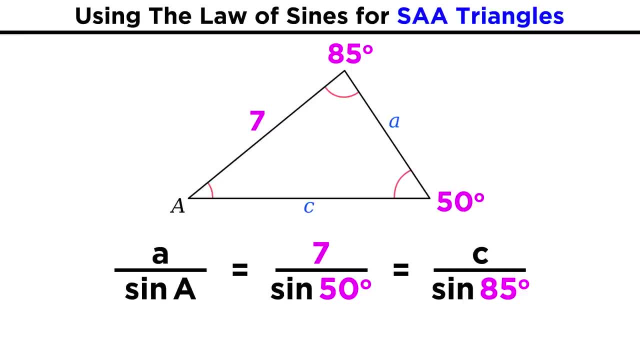 We can get the rest of the sides and angles using the law of sines. First, given two angles, we can always get the third. We just subtract these two angles from 180.. Now we have one angle-side pair, so we can use its ratio to get the other two sides. 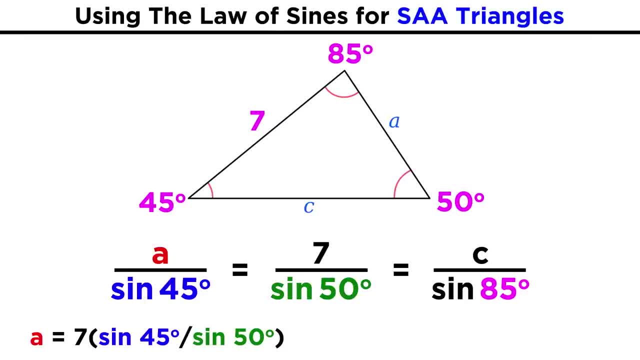 Here's one relationship. we just bring this angle up over here and then evaluate To get the third side. here's the other relationship and we just do the same thing. When we use this technique, we will usually measure angles in degrees and just plug things. 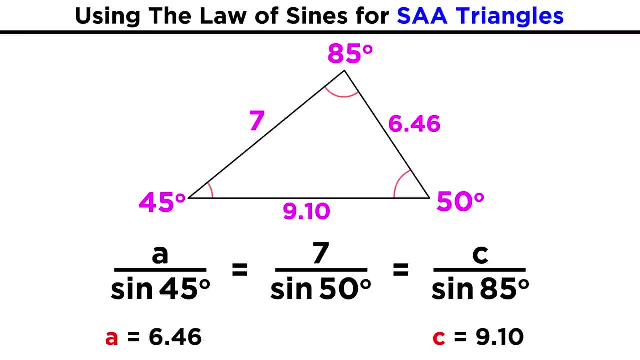 into a calculator to get approximate side lengths. Now that we've seen a side angle angle example, let's try angle-side angle. This is where the side we know is specifically the one in between the two known angles. In such a case we will again subtract the known angles from 180 to get the third. 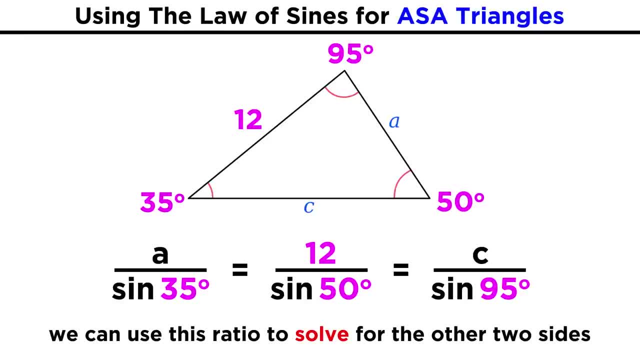 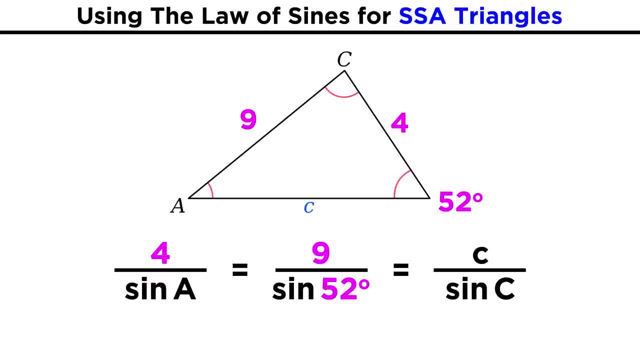 And once we have that, we are ready to plug values into the law of sines. Let's look at a slightly different scenario. Let's say we know two side lengths and one angle, which means side-side angle. Here we have to first find the angle opposite this side length.